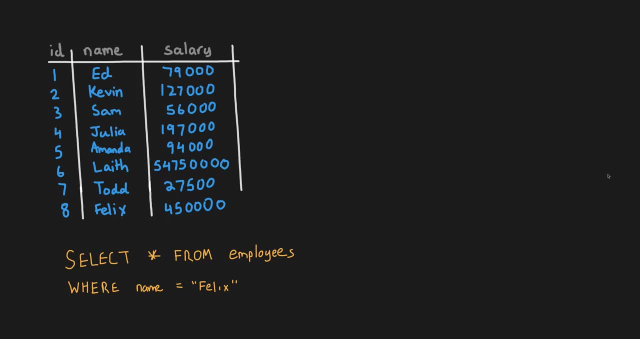 Let's say that you have an employees table in your database that looks a little something like this: So you have an ID column which contains a primary key, a name that contains the well names of the employees, and then the salary, which contains their corresponding salaries. And also, let's say that in your application you tend to perform queries that look a little something like this: So select star, select star means select every single column. 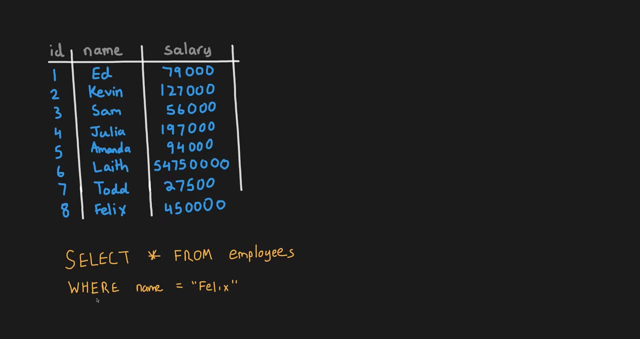 From the employees table and then we have a filter mechanism where we filter by the name And specifically for this query, we're filtering where the name is equal to Felix. So this query right over here should return this record. So where the ID is eight, the name is Felix and then the salary is $450,000. Okay, so that right. there is a very simple query. So let's actually talk. 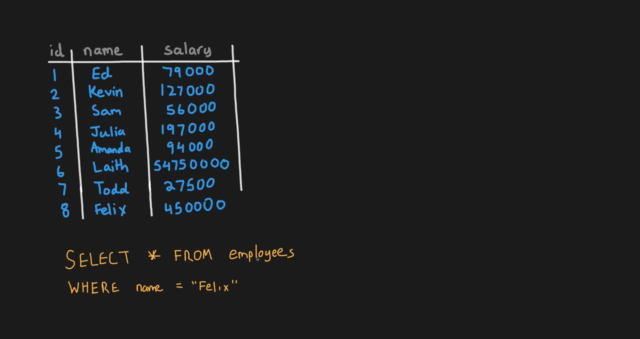 about how SQL actually gets that data under the hood. And you might be thinking that, well, okay, well, we have all our data in a table. you know, SQL probably just traverses everything and then finds where the name is equal to Felix, where we specified it, and returns those records. Well, you are correct, but you're also a little bit off. there's actually a little bit more complexity under the hood. So let's talk about that And then we can talk about how we can actually 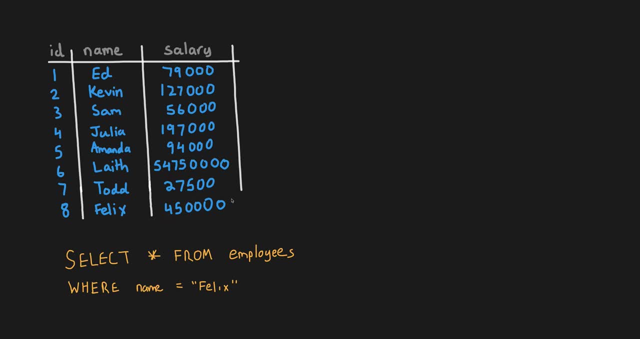 increase the performance of that a little bit later in the video, once you guys understand how SQL performs queries like this. So over here, essentially, you can see that these data are stored in this particular table, But in disk, in the actual databases, these records are stored in what are known as blocks. So blocks, you can essentially think of them as well, a block. 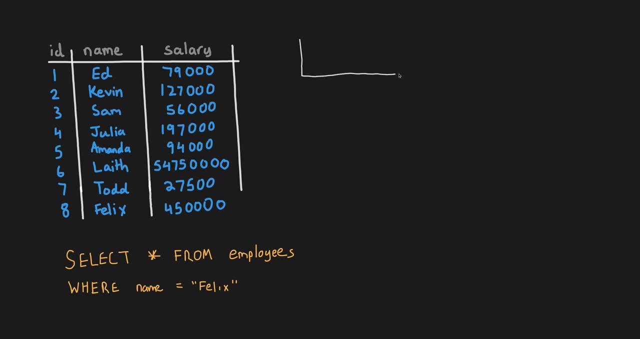 so that's a very kind of simplistic way of thinking about it. Well, a block right over here. we can have multiple blocks, and a block has a fixed amount of storage. For instance, in Postgres, the amount of storage that it has is eight kilobytes. Now, each block has a unique identifier, So we can basically give this block over here and an identifier of zero. Now, inside these blocks, we have all of our 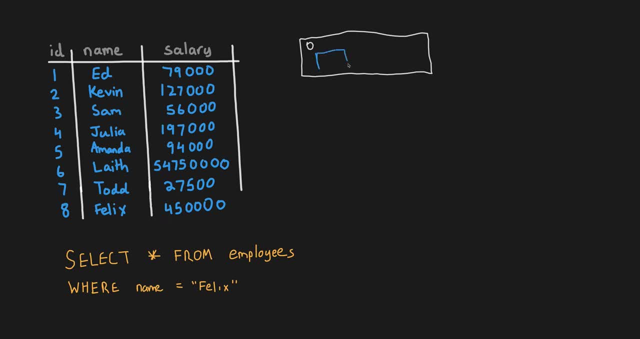 records. Now we can have something like Ed in this block. So we can have Ed in this block. So here's one record, And then we can have another record, Kevin, in this block. And let's say, each block, for our example, can only store two records. Well, for all the other records, well, they're going to be stored in other blocks. So they're going to be stored in other blocks. And so you guys don't have to watch me draw it. I'm just going to quickly pause the video and 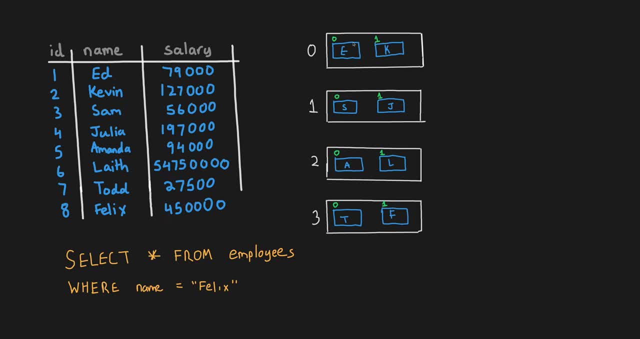 draw it out right now. So, as you can see here, the blocks contain a number of different records within them. Each block has a fixed amount of storage that it can persist. For instance, in a Postgres block, it can only persist up to eight kilobytes of data. So in this case, let's just say that each block contains two records. So over here we have Ed. over here we have Kevin. 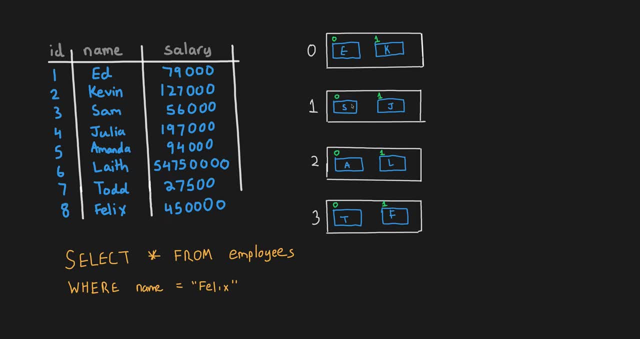 and then in this second block or block one, we have Sam, And then over here we have Julia. Now over here, in each record, this actually contains all of the information, And this is all of the information for each column, So the ID, the name and the salary. but for space reasons I only just put the name right over here. But this is basically how the data is structured inside of a typical database. Now, when you go to the database, you're going to see that there is an ăn. 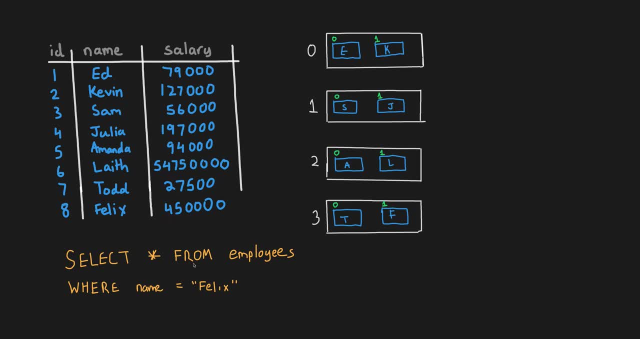 ahead and you want to perform a query like this. well, the database actually can't go ahead and parse every single record in each block. this block right over here or these blocks right over here are persisted in disk, so they're persisted in disk, the first step that the database actually has to 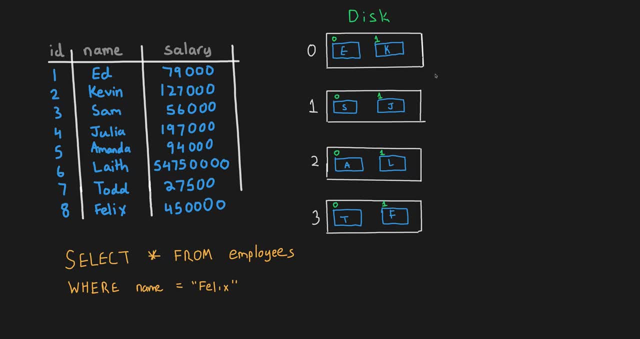 take is to essentially load up all of the records in memory. so, load up all of the records in memory, and this is actually not the best performance wise. however, this is what it has to do, so it basically has to take all these records and load them up in memory, ultimately resulting 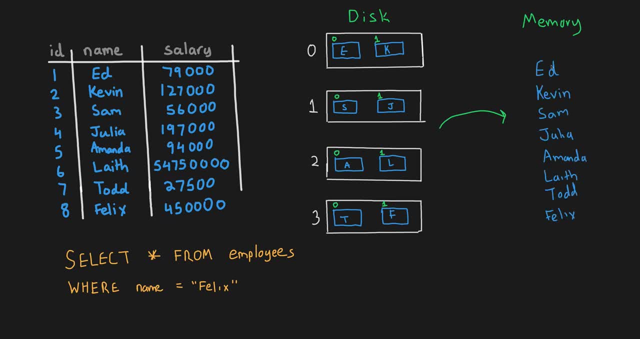 in something that looks like this. so, essentially, over here we have all of the records that were in the block, loaded up in memory. now, over here again, i have all of the names, but in reality it's going to contain all of the columns that we selected for. so here we selected. 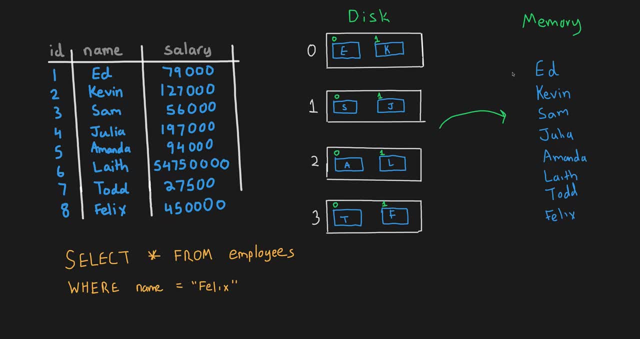 it for every single column. so in reality we would also have the id here and the salary, but just for space constraint i just put the name. now, once everything is loaded up in memory, the next step is to well traverse every single piece of information, every single record, and then essentially return back any record. 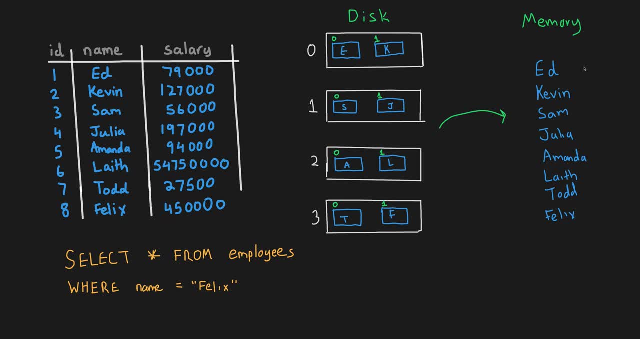 that meets this criteria. so now it has to essentially traverse all the records and for each record it's going to check if the name is equal to Felix. so over here it's going to go ahead, traverse this, and then it's going to realize: okay, well, this one's equal to Felix, so it's going to. 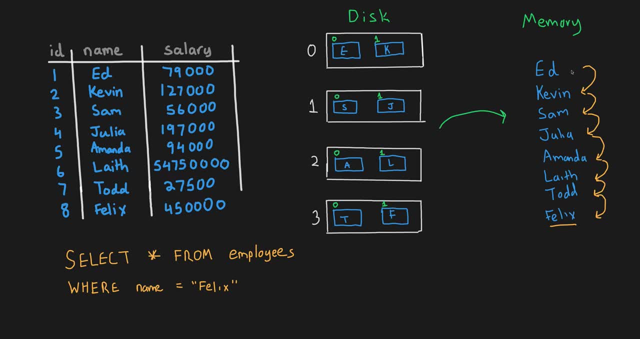 return this record. so if you know a little bit about time complexity, this is an O of N operation because we're traversing every single record inside of our database to get Felix to get essentially our desired outcome. so this whole process where we essentially take our data and 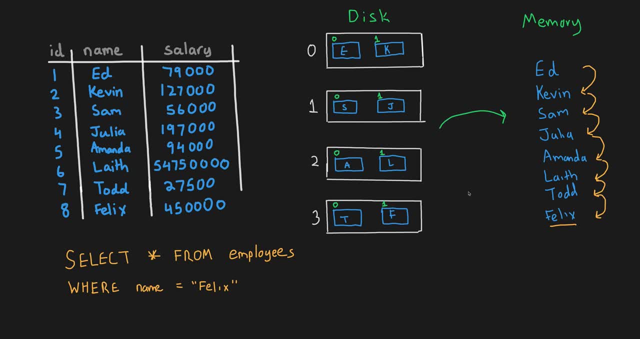 store it into or load it up into memory, which is very prof, which essentially takes a performance of the data and then it's going to return this record. so, if you know a little bit, and then traversing every single record until we find all the records that meet our criteria. 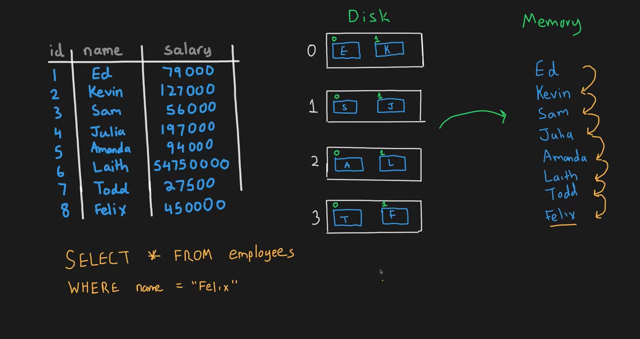 is known as a full table scan. so full table scan, and for the most cases, full table scans, are not that performant. now, in this case, well, when we only have eight records, it's okay that this is completely fine. but what if we had, I don't know, five million records, ten million records? what if you had an application like: 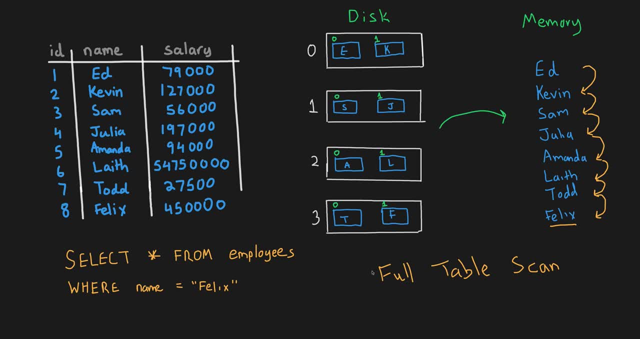 Twitter, where we had billions of records. a full table scan can get very, very, very slow. so how can we improve this? well, we can improve this with indexes. so I did a little bit of erasing, because the way that we query our data with indexes is going to be a little bit different. 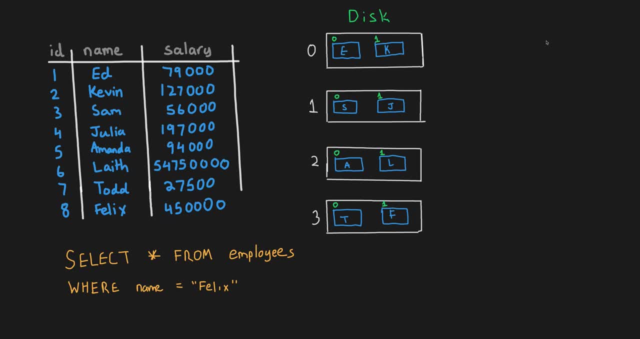 than you know, putting our data in memory and just iterating through it. so, essentially, with an index, the first thing we have to do is put our index for a specific column inside of our database and this column is going to be essentially a column where we use a lot to query our data. for instance, in this example we use the name column quite. 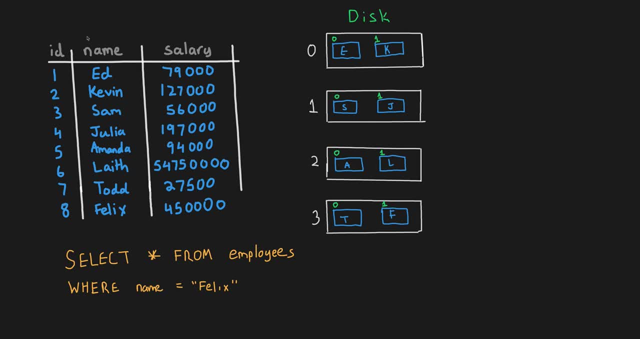 frequently to query our data, so we're going to probably want to put the index on this name column. so if we go ahead and do that, so let's say we go ahead and there's just a simple query that allows us to add an index on a particular column in the table. essentially what happens. 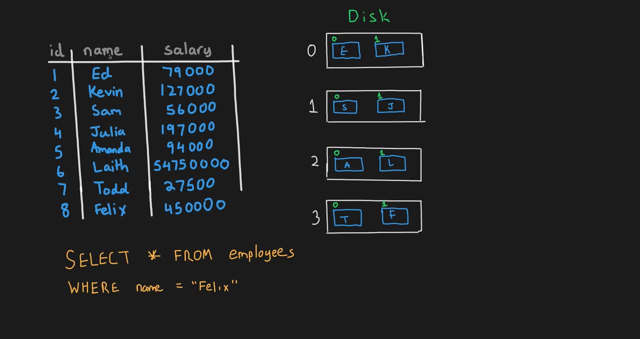 behind the scenes is that the database creates a brand new data structure that looks a little something like this right over here: give it some time, it should render. it's not rendering, unfortunately. let's give it a little bit more time, there we go. so it looks like this. so this is essentially how. 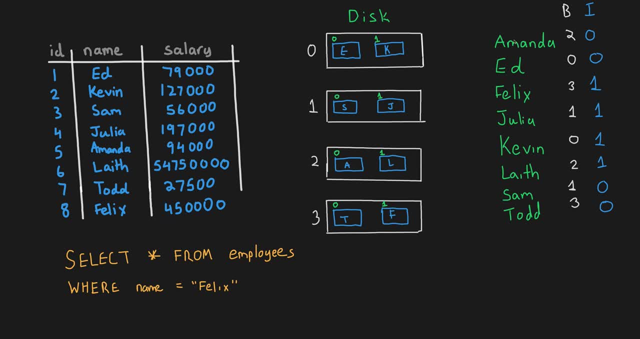 this is going to look. so, as you can see here over here, we only have the names, so we don't have the salary, we don't have the id, we only have the thing, the column that we actually ended up indexing, and along with the name, we actually have two pieces of information, essentially these two pieces of 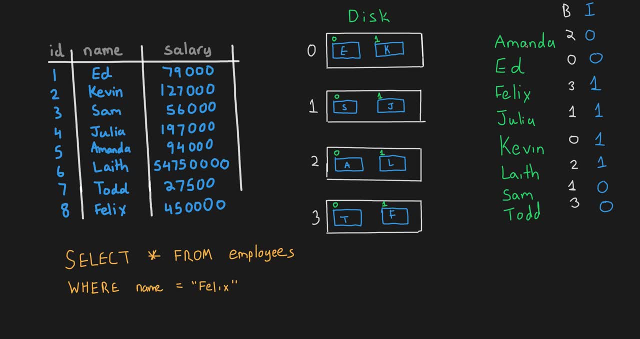 information. you can think of them as location coordinates. so over here you can see that we can see that amanda is located in block two, index of zero, inside of that block. similarly with felix, okay, that's located in block three, index of one. so this is a brand new data structure. 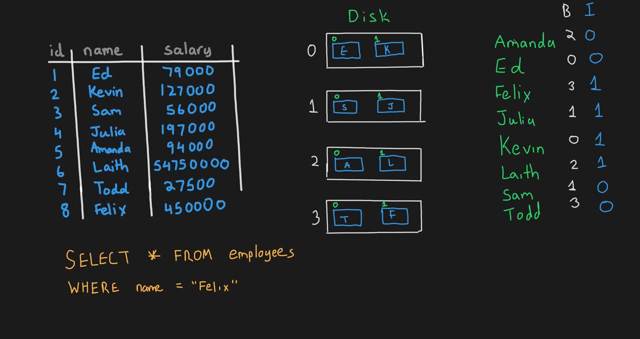 that is actually stored inside of the database. now the data structure doesn't really look like this, like this kind of list. actually, what it is is kind of a b tree, that's the most famous index, but for the sake of simplicity i'm just going to keep it kind of this linear line. so over here we. 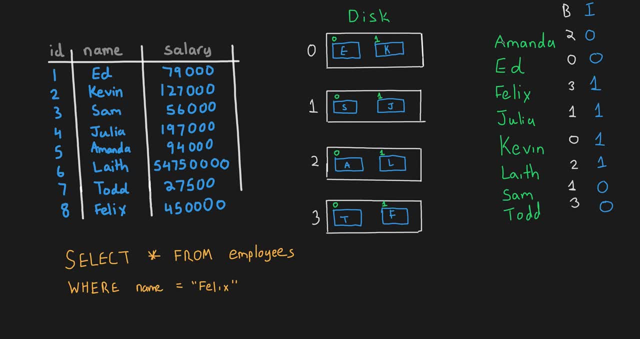 have this data structure right over here and you can also see that this data structure is not in the same order as basically the names inside of this table. you can see here that you know we have amanda in the beginning, then we have ed, then we have felix and then we go all the way to todd. 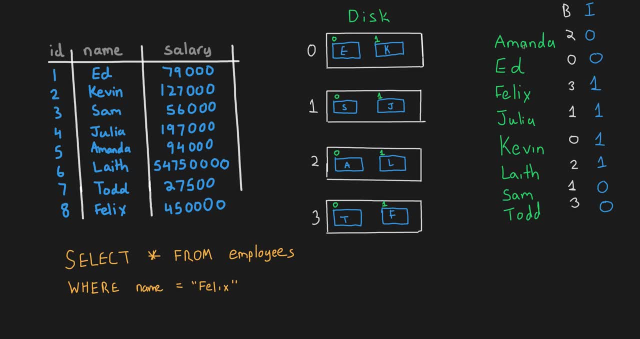 and essentially this is ordered in alpha and then we have amanda in the beginning and then we have amanda in alphabetical order. it's actually sorted in some way, and this is very, very important, because things that are sorted are a lot faster to query, and let me kind of explain why. so let's say we 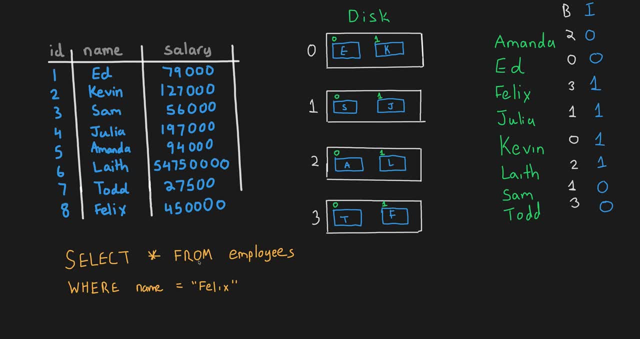 perform this right over here. we perform the same exact query instead of iterating through everything, or instead of actually going to the disk, putting it into memory and then iterating through everything, and then we find felix, a full table scan. what ends up happening is it goes to this index that we 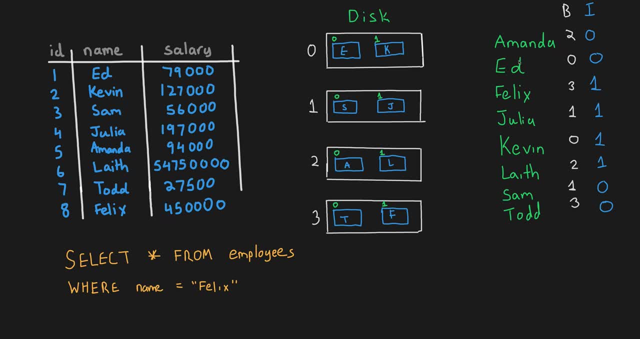 created this brand new data structure and basically what it does, is it okay? so it checks: essentially is felix. is felix greater than or less than essentially the middle of this index right over here? so in this case it is less than from an alphabetical standpoint. so it goes ahead and it completely neglects all of this, so it doesn't even have to iterate through. 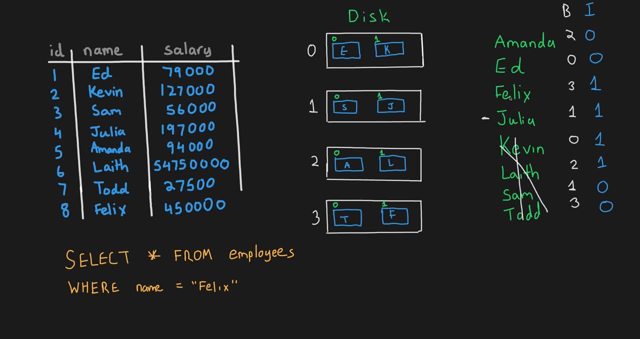 all of this and then it goes to basically the next middle. so over here you, you can't really figure out which one the middle is. let's say ed is the middle. so in this case we can say: okay, well, is felix greater than or less than ed? well, in this case it's greater than, from an alphabetical perspective. 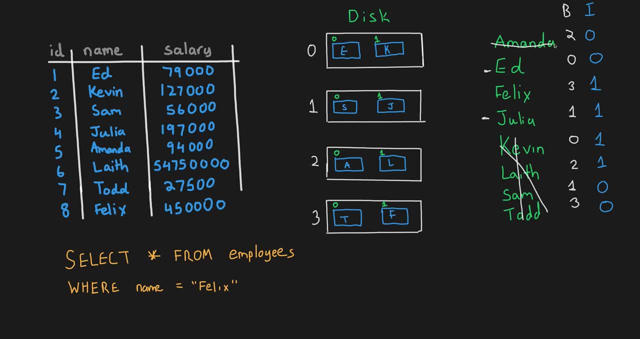 so any any date over here we neglect it. so right here we have one, but you can imagine we can have millions of other records, we can have millions of other records, we can have millions of other records, and then we do this so on and so on, until we filter for felix and over here we only have one. 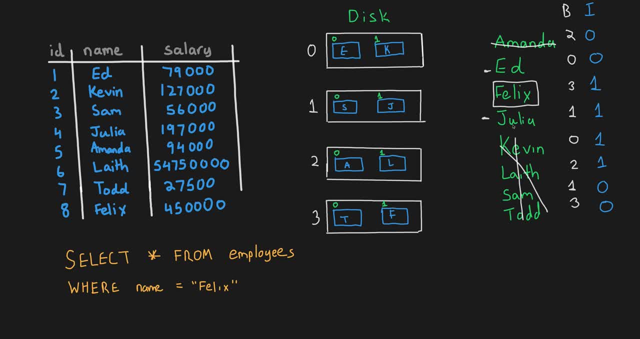 felix. but there is a possibility that we have multiple felixes, so we can just have that kind of iteration process to basically get all of the felixes and then we would also get their corresponding block and index, and then once we do that, we can essentially get the block and index. 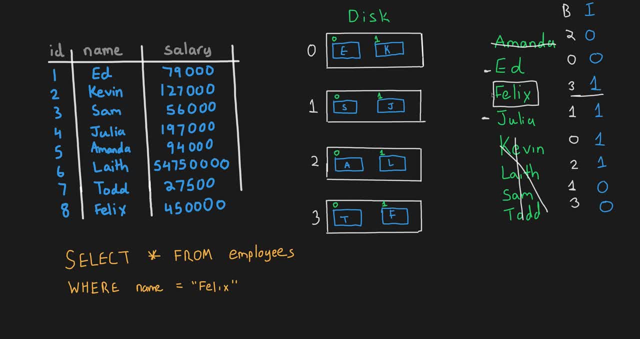 and instead of loading all these things into memory, what we can do is we can essentially go to block three and then index one, which is right here, and get that data and end up returning that data and remember that data contains all of the records, the id, the name, 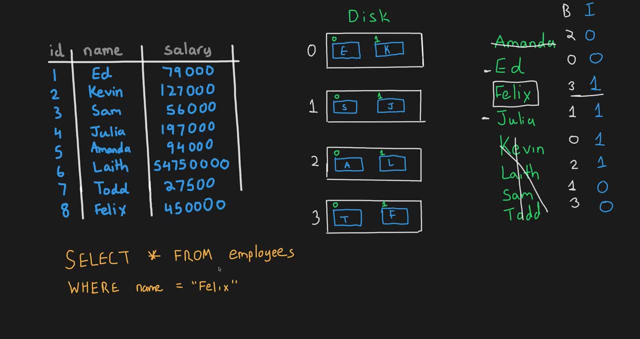 and the salary. so that is significantly faster now. why is that faster now? remember the reason why it's faster is because we're essentially halving our data set with each iteration, so we're not going to have to do that in every single one. through each one, we're halving our data set. 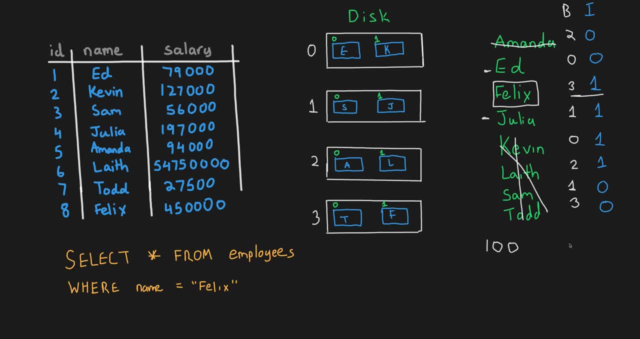 so, for instance, if we have maybe 100 records, the first iteration we would completely get rid of 50 records. so now we only have 50 records that we want to worry about instead of parsing the whole 100, then we would parse, basically we would parse these 50 and then for the next iteration we would 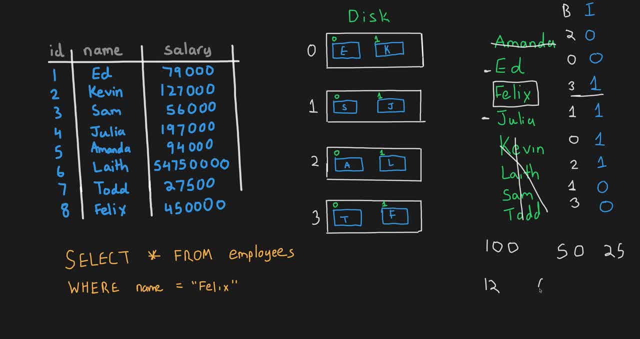 worry about 25 records and then 12 records, and then six records and then three records and then say one record. so you can see here, this is one, two, three, four, five, six, seven, seven iterations versus 100 iterations, and you can see why indexing is so much faster than just you know. 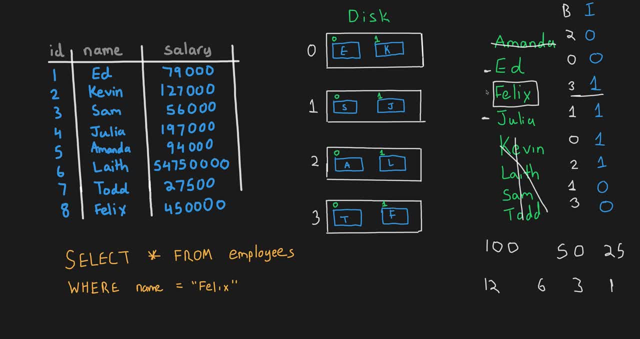 just basically putting everything into memory and then parsing it, because there we would actually first of all have to put everything into memory, which is expensive, and then parse every little thing, which would take 100 iterations. now this is known, if you know your time complexities, as log n time and this is kind of an ideal time complexity, and this is really known as a binary. 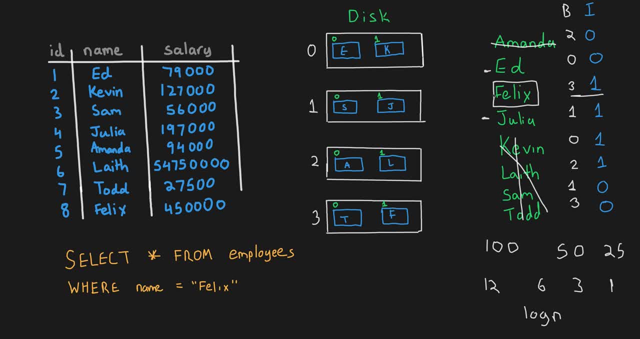 search, and this is why this is going to be organized as a tree in the database. but for simplicity's sake and because i don't have much space in the board, i just kept it like this. but this is stored as a tree rather than a kind of linear list. all right, so cool. that's, that's pretty. awesome and that right there kind of explains you the way that we're going to use indexing in the database and that's kind of the way that we're going to use indexing in the database and that's kind of the way that we're going to use. 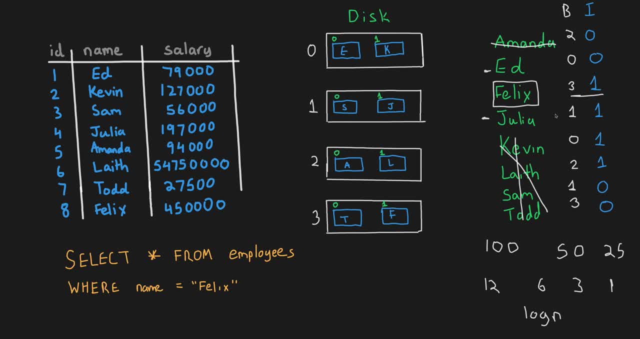 why you probably want to add indexes to speed up your queries. Now there is one thing you might be thinking: okay, let me just add an index to everything. Well, that might not be ideal because, yes, indexes they do speed up your queries. However, you're storing all this extra. 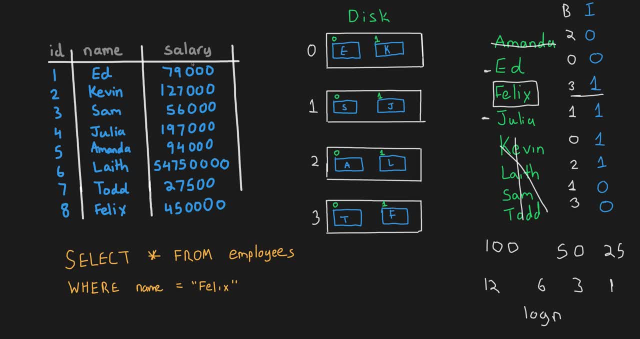 data. So you're storing actually a lot more data. And remember, if you have millions of records, well this is going to be kind of a million long- we're going to have the column name and their corresponding block and index. So that is one thing that you have to worry about. So you probably 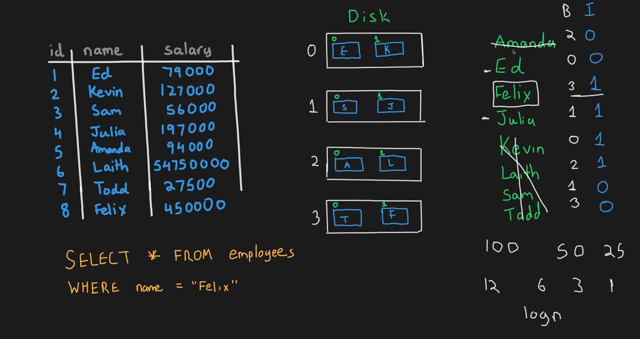 wouldn't want to add an index to a column that you don't really query by, because you're adding additional data And you know if you're working with a production application, additional data is going to cost you money. Now, another thing is that indexing can actually lead to performance. 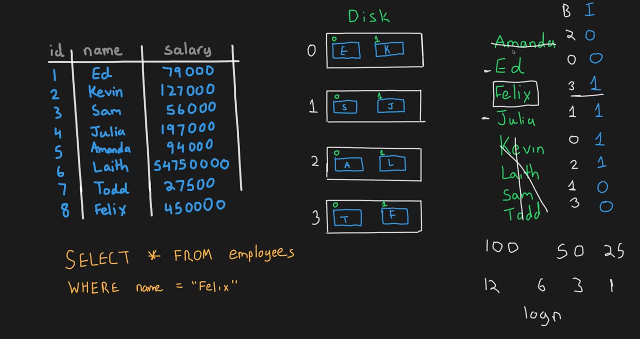 hits. So, for instance, if you are updating your data a lot, if you are writing data a lot, well, you're going to have to write this data or update the state of the data inside of the table itself, as well as the index, And 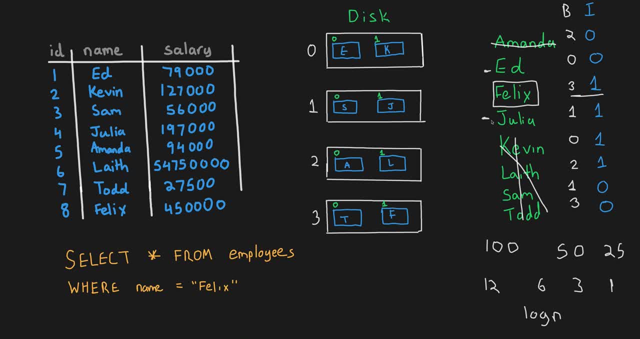 this is well less performant as not having an index. So you really have to think about when you want to actually index. and I prefer to index something if I'm by index a column, if I'm using it quite frequently, from basically filtering by that comment but by that column quite frequently. 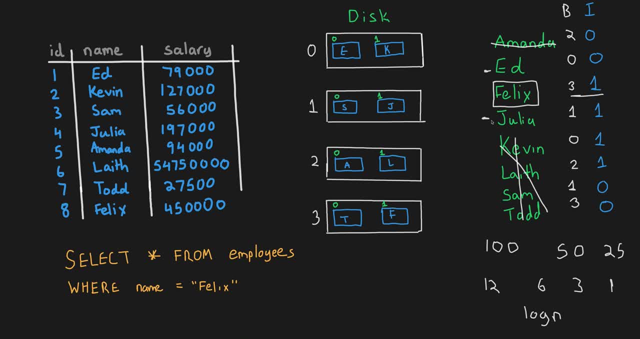 and I'm not really adding or updating or deleting records in that table as much, And that's what I tend to like to use indexes because they just speed up the process And I don't have to really worry about the performance hit that I get from inserting data or updating data or even deleting data.